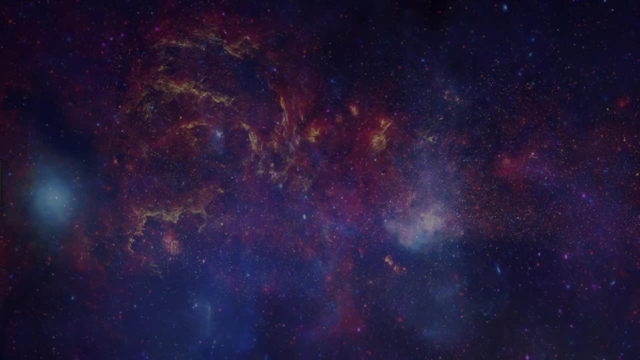 the weights And it does this process over and over again until it's found a minimized loss. We cover how this update is actually done using the learning rate in our previous video. that covers how a neural network learns. So when SGD calculates the derivative, 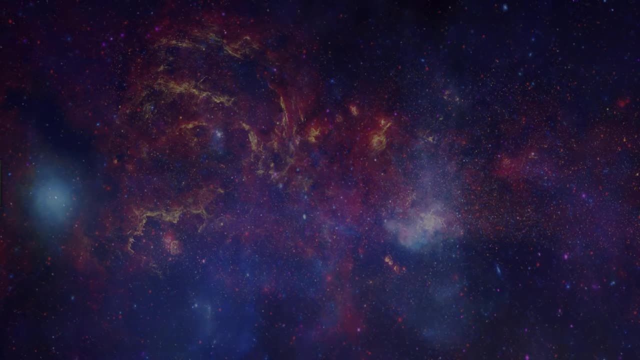 it's doing this using backpropagation. So essentially, SGD is using backprop as a tool to calculate the derivative. So when SGD calculates the derivative, it's doing this using backpropagation. So when SGD calculates the derivative, it's doing this using backpropagation. 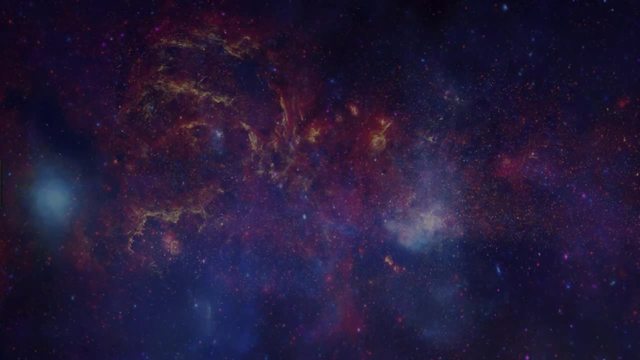 Going forward. this will be our focus. All the math that we'll be covering in the next few videos will be for the sole purpose of seeing how backpropagation calculates the gradient of the loss function with respect to the weights. Okay, we've now got our refresher of backprop. 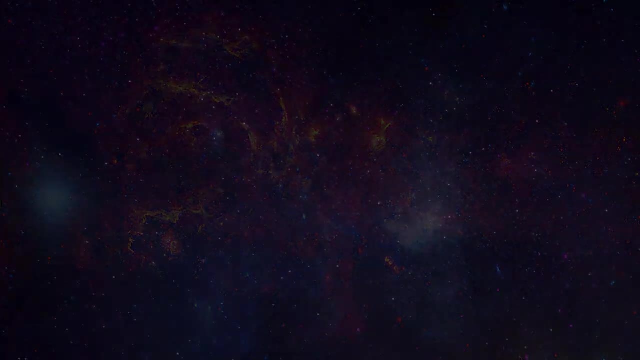 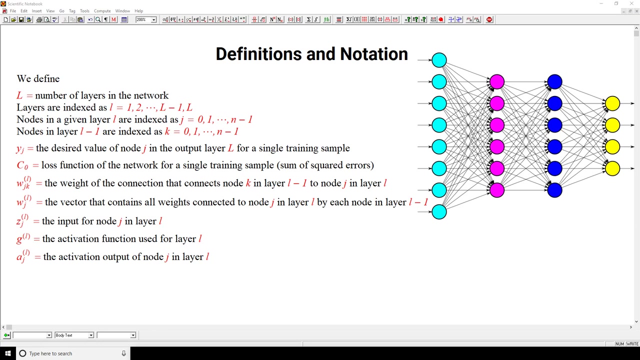 out of the way. so let's now jump over to the math. Alright, I'm going to have to go full nerd on you guys and pull out my mathematics scientific note book that you see on the screen here to show everything properly. We're going to start out. 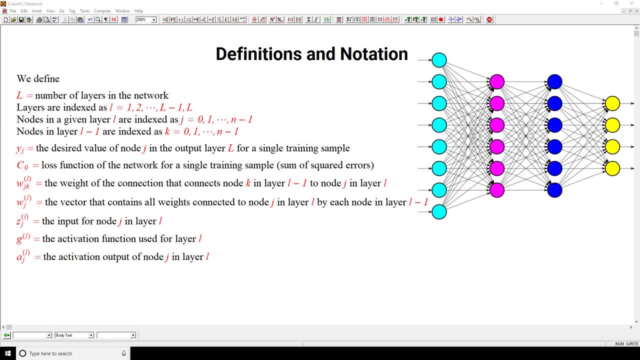 by going over the definitions and notation that we'll be using going forward to do our calculations. So let's get started here. We start out by defining big L as the number of layers in the network. Layers are indexed sequentially as L equals 1, all the way up to big L. 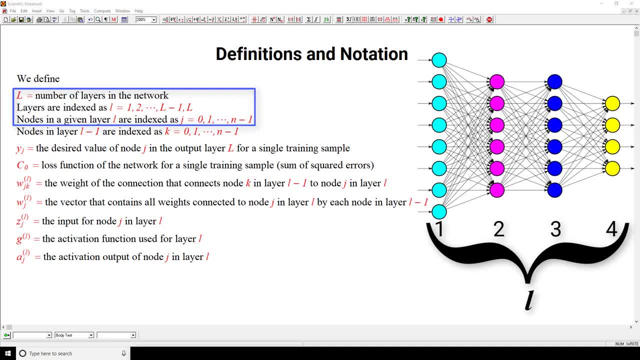 The nodes in a given layer L are indexed as J equals 0 all the way up to N minus 1.. And the nodes in a previous layer, which would be L minus 1, are indexed as K equals 0 up to N minus 1.. When we're referring to a layer L, 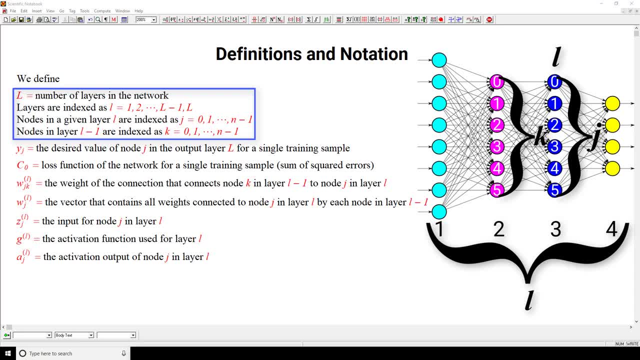 the indices that we're going to be using to refer to those nodes are going to be J indexed, And when referring to the layer L minus 1 that's directly preceding L, the nodes in that layer are going to be K indexed. So, moving on to the next definition, we then define Y sub J as the desired value of node J. 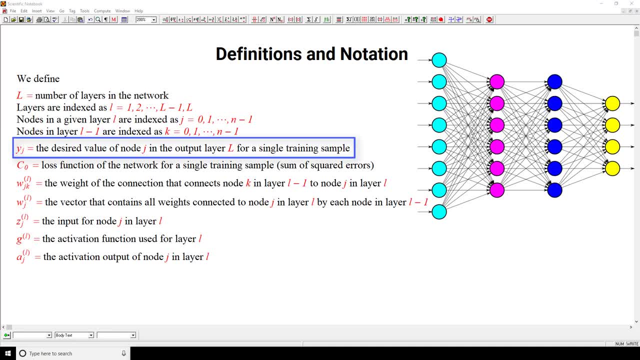 in the output layer big L for a single training sample. So given that we have labeled training data, we know ahead of time the output that we desire for any given input. And so Y sub J here is the desired value of some given input. 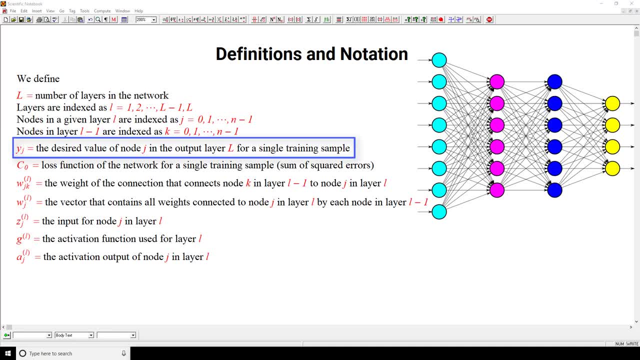 for a particular node J in the output. So we're going to define Y sub J as the desired value of some given input. So we're going to define Y sub J as the desired value of some given input. Next, we define C sub 0 as the loss function of the network for a single training sample. 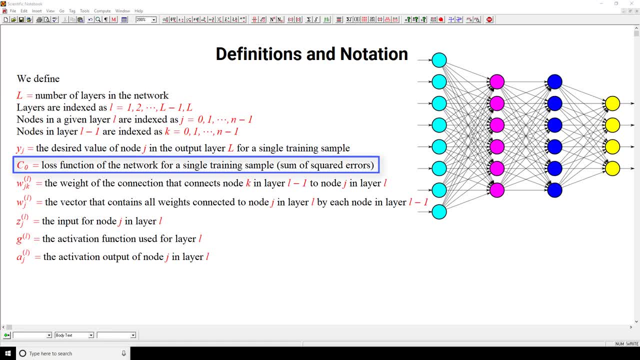 which is going to be the sum of squared errors here, And actually, just like in our previous video, our discussion here is mostly going to be focused around passing one single training sample into the network at one time and seeing how back propagation works in that regard. 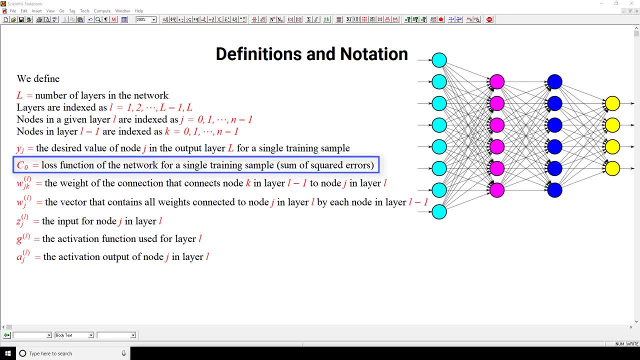 And then the logic that we build up here will be able to generalize to when we pass more than one training sample at a time. Next we have W sub JK superscript, small. l Note that this is a superscript, it's not an exponent, And this is equal to the weight of. 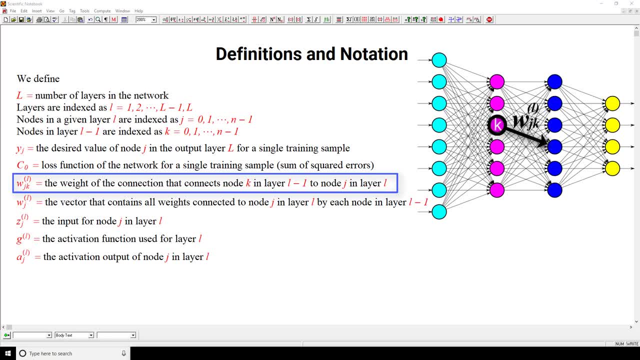 the connection that connects node K in layer L minus 1 to node J in layer L, And you can see that in this illustration here. Next we define W sub J, superscript small l, And this is the vector that contains all the weights connected to node J. 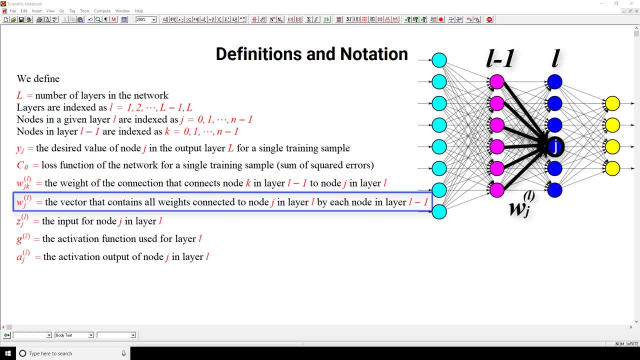 in layer L by each node in layer L minus 1.. So we can see by our illustration here how this definition differs from the last one that we just defined. The last one was for one specific weight that connected two nodes in two separate layers together, And the definition that we just gave. 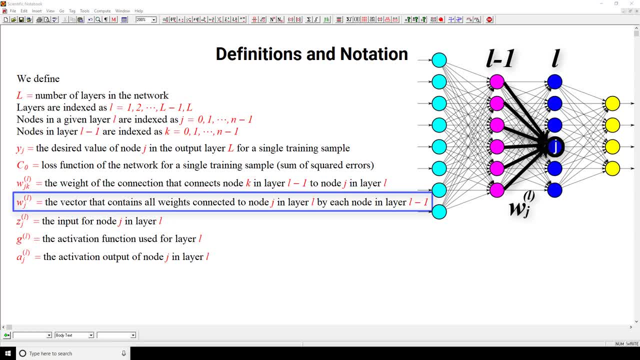 is an accumulation in vector format. So we're going to define W sub JK, superscript small l. That contains all the weights connected to this specified node J in layer L by each node in the previous layer, L minus 1.. Moving on, we now define Z sub J, superscript small l, as the input for node. 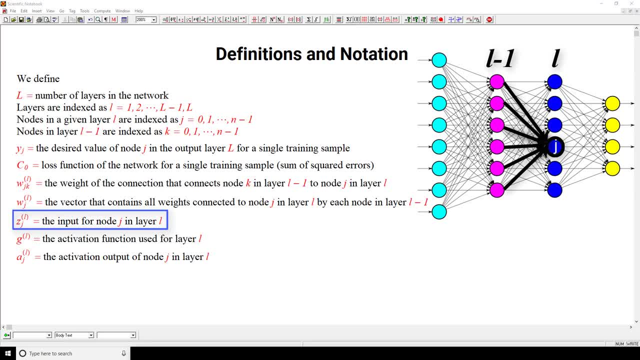 J in layer L. We know that each node within a layer receives a weighted sum of input from the previous layer. This weighted sum is being represented by this Z sub J superscript L here. Next we define G superscript L as the activation function that's used for layer L. 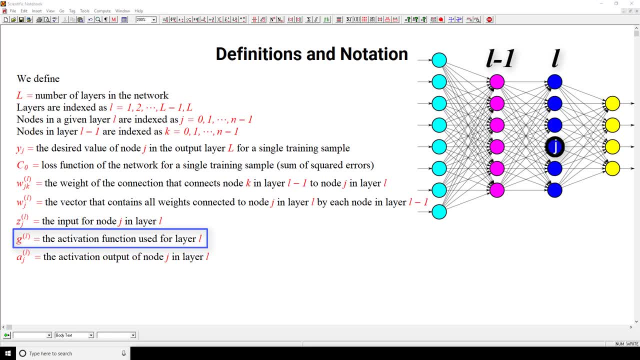 So after a node receives input like that that we just defined in the previous definition, it's then going to pass this input to an activation function And we're using this G superscript L here to represent that activation function for a given layer L. 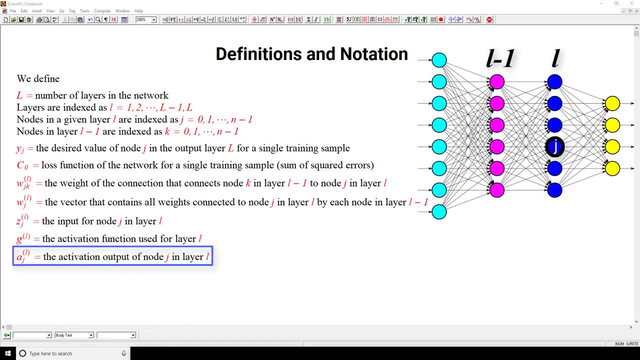 And finally, we define A sub J superscript, small l, as the activation output of node J in layer L. So what do we get after we pass our input from a node into the activation function? That's going to be the activation output that's then passed on to the 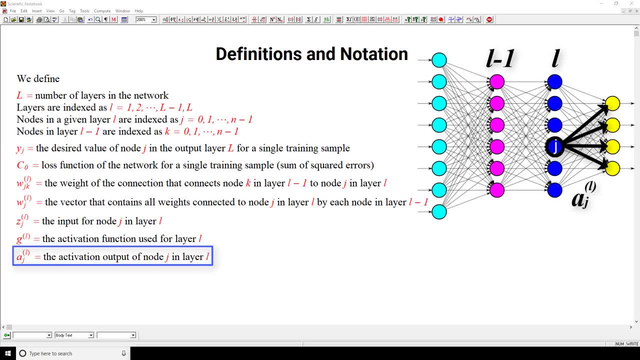 next layer, And so we're representing that with this A, sub J, superscript L here. Alright, so these are all the definitions that you need to know before moving forward. Now let's narrow in and discuss the indices used in these definitions. 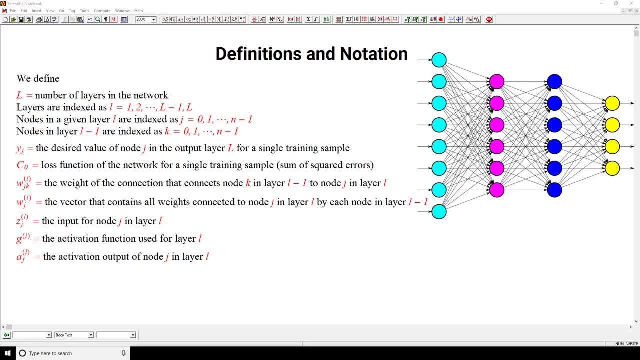 a bit further Recall. at the top of our notebook we covered the notation that we'd be using to index the layers and nodes within our network. All further definitions then depended on these indices. We saw that for each of the terms we introduced, we have either a subscript or a. 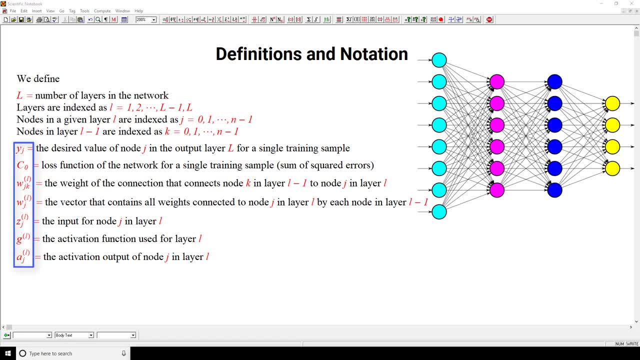 superscript or both, And sometimes our subscript even had two terms, as we saw when we defined the weight between two nodes. So these indices that we're using everywhere may make the terms look a little intimidating and overly bulky. That's why I want to focus on this topic further here. 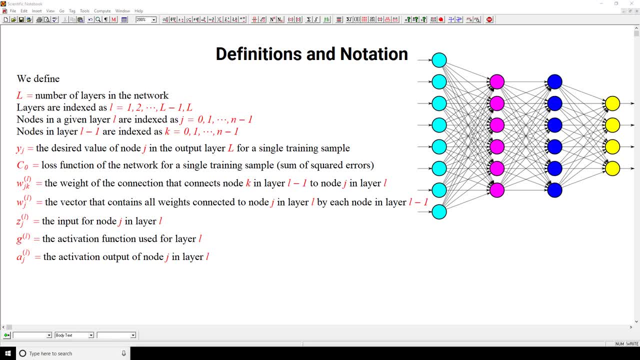 It turns out that if we use these indices properly and we understand their purpose, they're going to make our lives a lot easier going forward when working with these terms, and will reduce any ambiguity or confusion rather than induce it. You may be familiar with in code when we run loops. 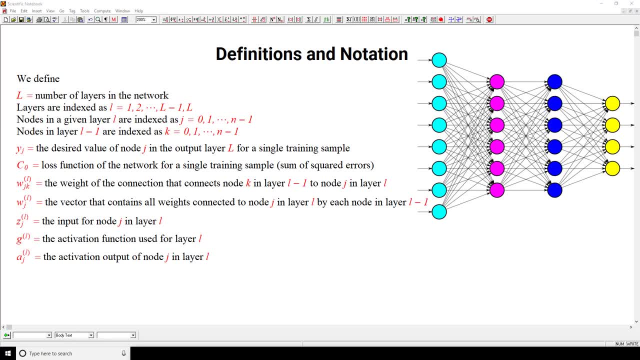 like a for loop or a while loop, that the data the loop is iterating over is the same as the data the loop is running in. This is an indexed sequence of data. Indexed data allows the code to understand where to start, where to end and where it is at any given point in time within the loop itself. 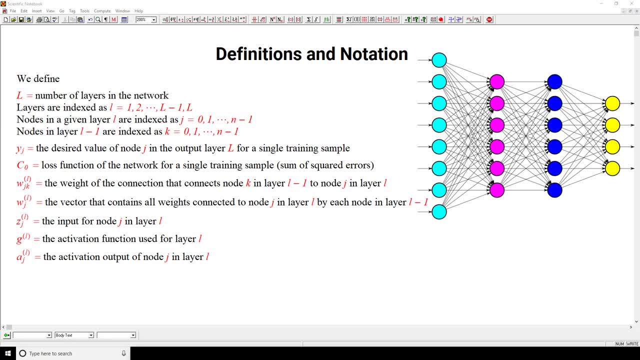 This idea of keeping track of where we are during an iteration over a sequence is precisely why keeping track of which layer, which node, which weight or really which anything that we introduce here, is important In the math in the upcoming videos of iteration, particularly via summation, where summation is simply the addition.